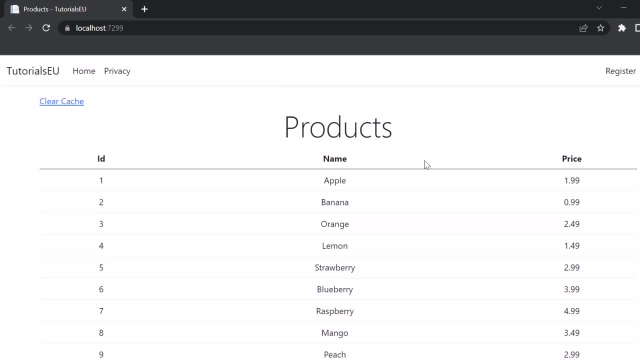 it will get loaded Super fast because it's cached in the memory of the server. So right now everything is cached already. We will just dig deeper into how it works exactly just in a second. But if I now clear the cache and the page automatically reloads, for sure the data will get fetched from the database. 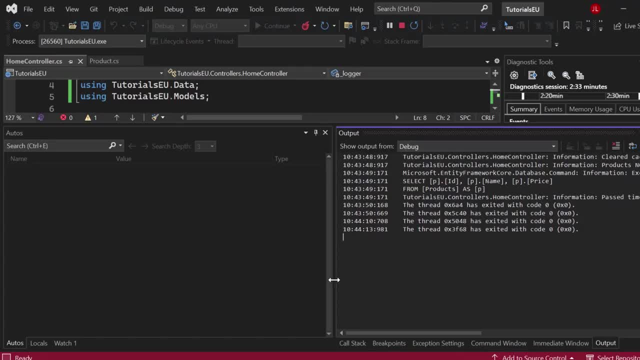 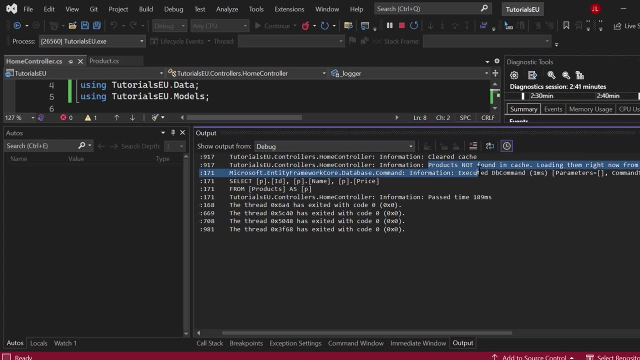 So let's take a look at our application right now. I got some pretty nice logs right here. You can see that after I clicked on clear cache here, we got it right on screen, it got loaded from the database again and it took in total 189 milliseconds. Now, right now. 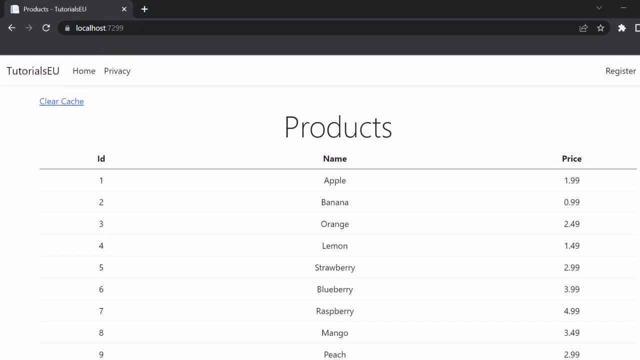 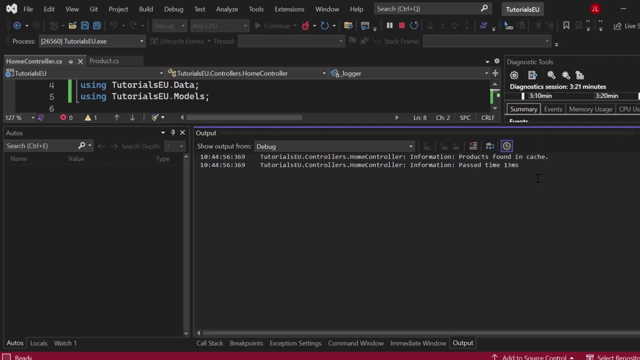 everything is cached again. So when I simply reload the page and now go back to our logs, you can see that it only took 13 milliseconds right, And it differs. Sometimes it's two milliseconds. Right now I got a screen recording program and all of that running. 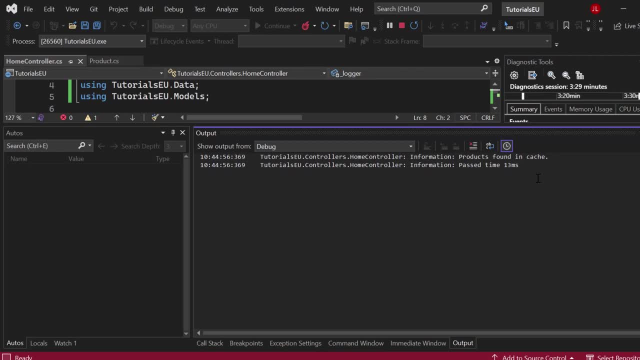 And sometimes it's 10 milliseconds, but it's definitely way faster. It's so much faster, Well, just think of it like 10 times, 50 times or even 200 times faster. Well, loading from cache is definitely something that you don't want to miss, So let's find out how. 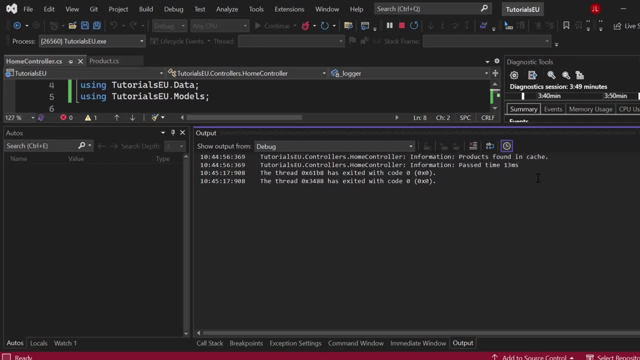 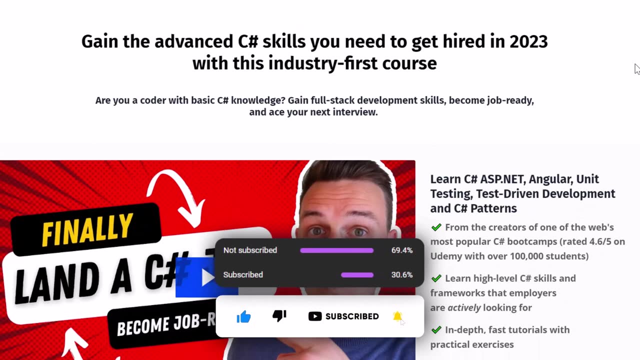 to get to your ASPNET Core application, And I can promise you it's way easier than you think. But first of all, make sure to subscribe to our channel so that you no longer miss any upcoming NET related videos, because we are here to help you become a better developer, And for sure. 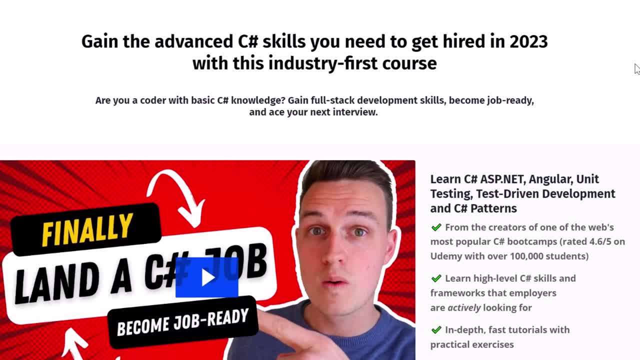 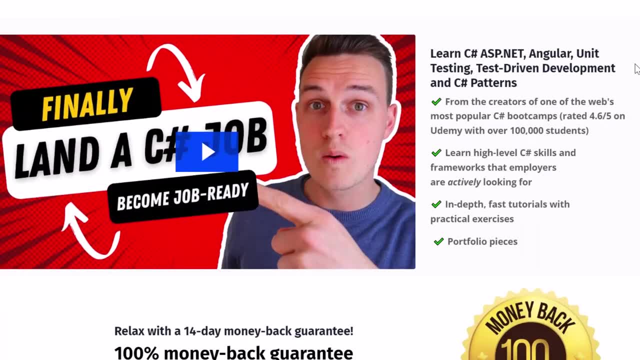 you are interested in that, Also, smash the videos like button. if you love ASPNET And if you take your C Sharp Curious series, check out our C Sharp Progress Academy. It's a self-paced online course turning you into a full-stack C Sharp web developer with 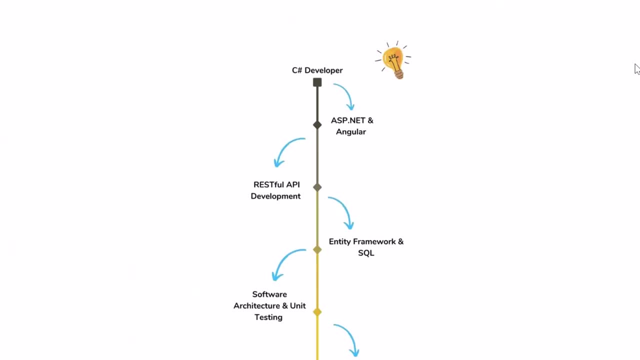 Angular ASPNET Core and I can promise it's the fastest way on how you can progress as a C Sharp developer. You can find the link in the description below or popping up right now at the top right corner. Now let me just shut down the application. We will. 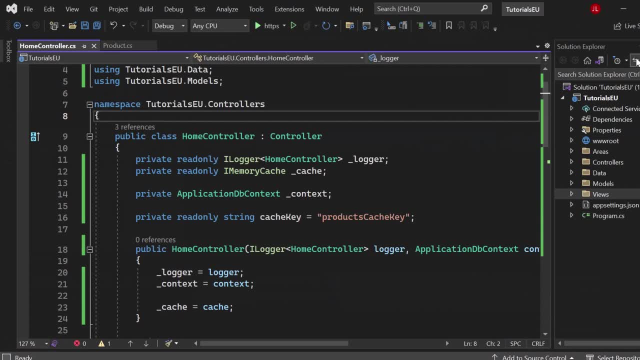 get to that just in a second again. Now let's get started. I will close everything here. Now let's talk about caching. So first of all, the good news is, as long as you use kind of MVC or any of the other templates on ASPNET Core, that gets provided. 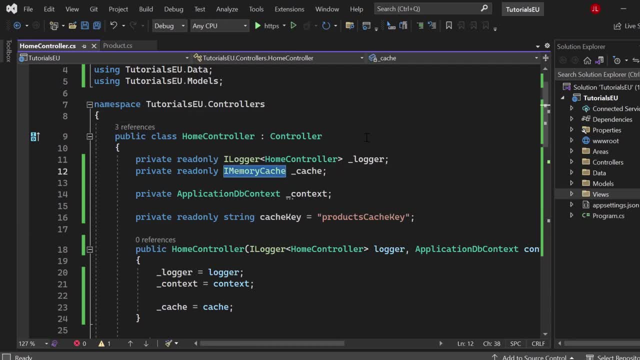 you can just use the I memory cache. It automatically gets injected via the dependency injection. Now, if you have no clue about the dependency injection, check out our video on that topic, Since it's really important if you are a NET developer. 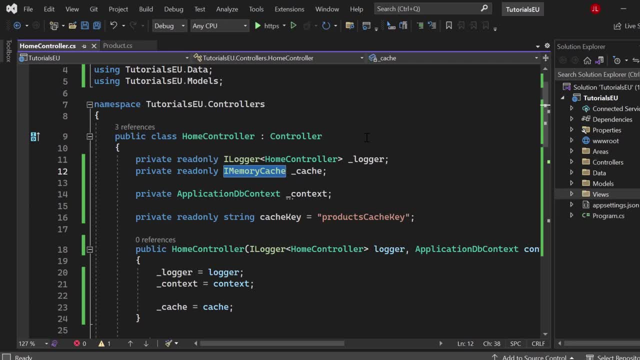 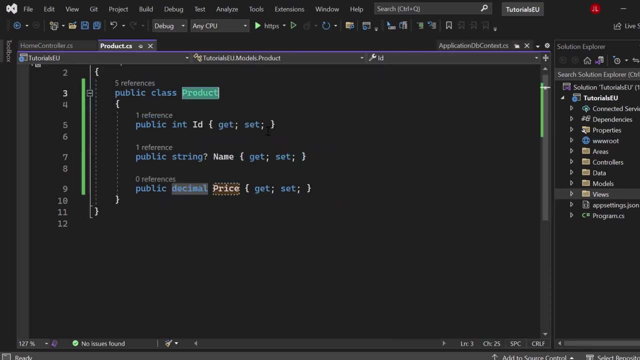 you have to understand how services get injected into your applications. Great, Now, afterwards, what we have right here is simple, very simple MVC application. We have an application to be context right, So nothing special. inside here We got the products, and the product consists of ID, name and price. but that doesn't really matter. It could be really. 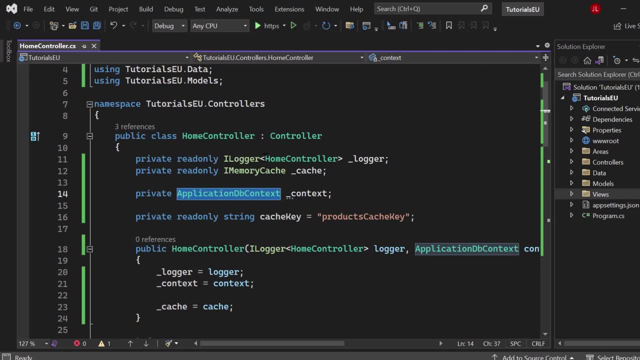 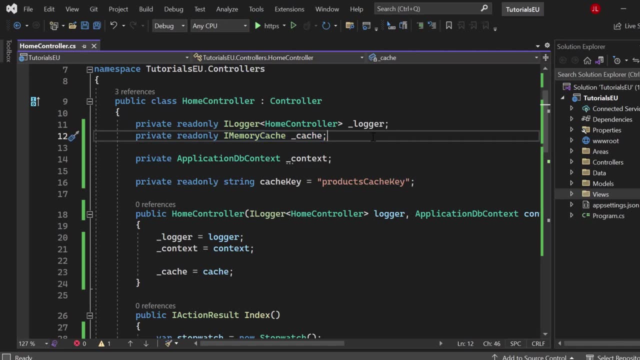 anything Great. So let me just close that again. I just want to show you the code here Now. what we have right here is an I memory cache, So that's quite important. You need that And, as I said, you don't have to install any additional package. It gets automatically provided. 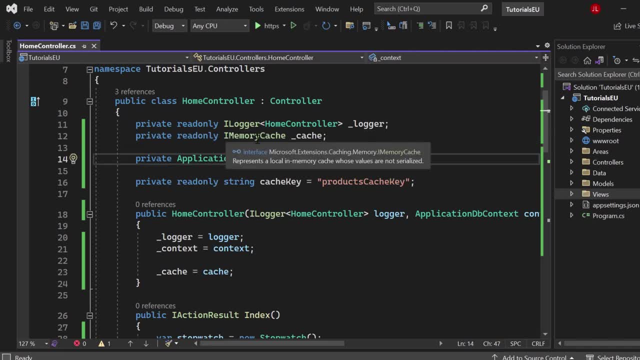 Now, as the name already indicates, it is saving the cached items to the application's memory on the server side, not on the user side. We are not talking about any kind of user cookie. No, we are saving the products inside of the server memory cache, so that, let's say, user A 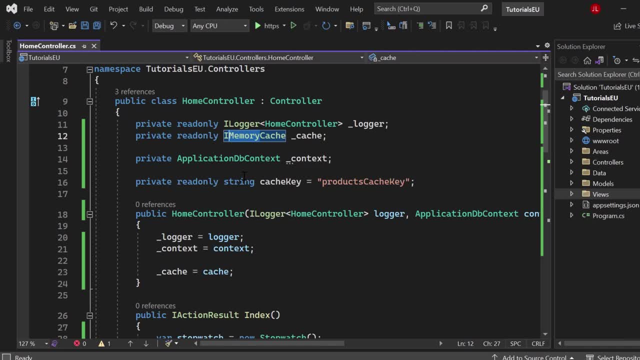 is requesting the products, Now it gets saved on the server. Now user B wants to get them too, And the cache data just gets transferred to the user right. So just keep that in mind. The cache data is lying on the server, not on the client side. Now here we got a cache key. Well, 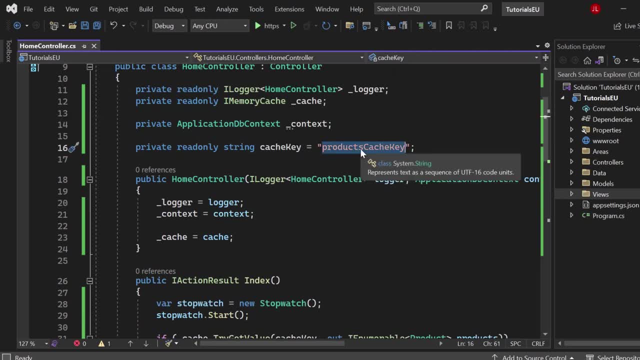 that's just kind of like a dictionary key right. So you have any specific key for any specific key. We could have a user cache key, products cache key, whatever Invoices cache key. Maybe not the best idea, but it would work. So you have a key. That key is connected to cache data. Well, 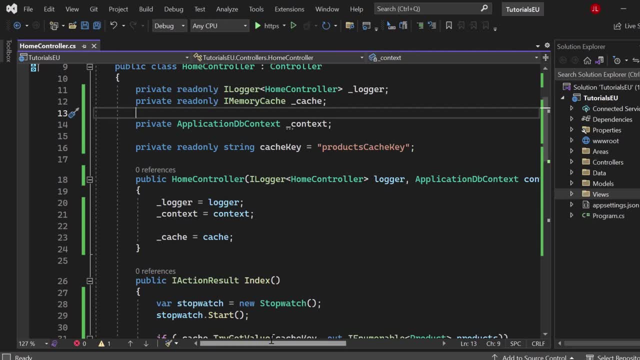 maybe. Now, here we got our constructor, And that constructor is just taking that I memory cache from the dependency injection so that we got an instance from it. Awesome, And now let the magic happen. right Here we got our index page, which is just as I said. it's an MVC application. It 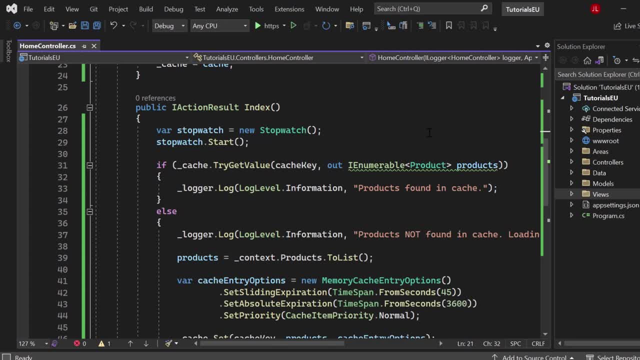 just shows our index page, that huge list of products. Now let's see what we can do here. So what I do right here is just creating a stopwatch so that we can measure the well actual time that's passing from starting the request to finishing it right now. Here is where. 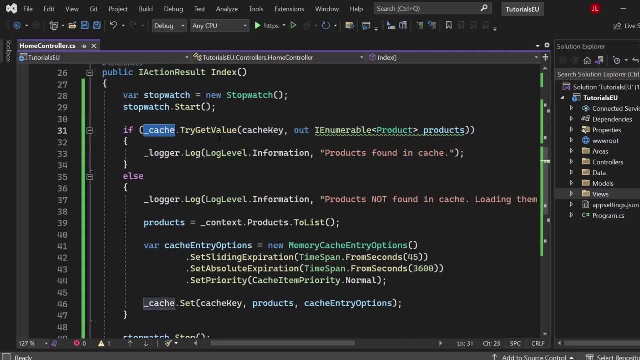 the real magic is happening, right. We are using our cache object. We are trying to get a value. You know that. try get value right. It's a method that you use when you work with dictionaries. Now we submit the key here, So we say, Hey, try to get a value from the cache. 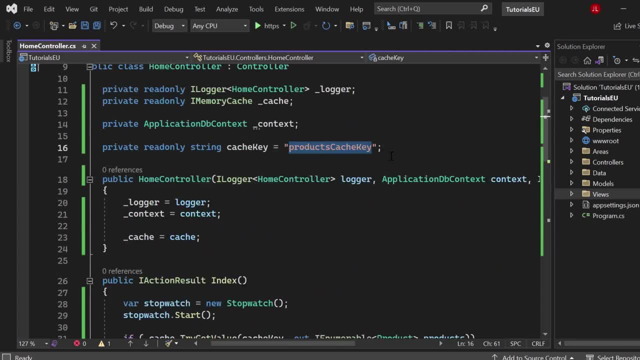 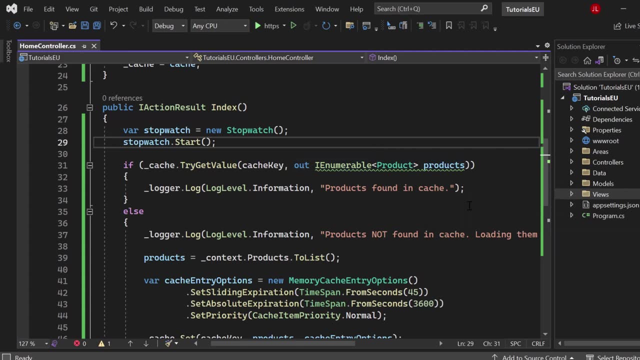 Using the cache key, which is, as I said here, the products cache key. it's just an identifier, And then we maybe get out our products as an I number. Now, if we do as I said, we put them out. 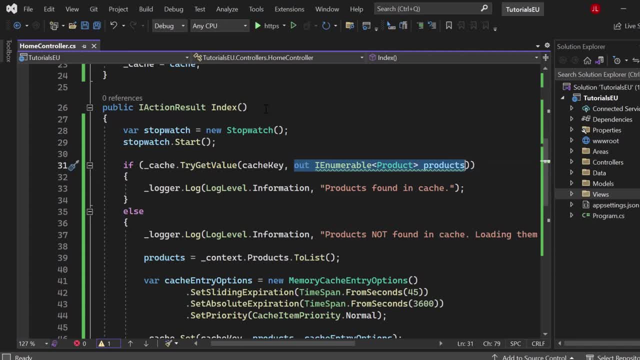 So they are available in the scope of the index method. If we have them in the, in the key, because we're using, if we have them in the cache, because we can use the out here Now we also lock something: products, fountain, cache, right, Awesome. And if we don't have them in 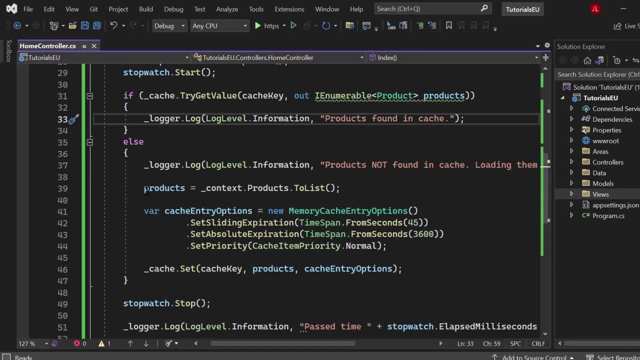 the cache we can see products, not. So we simply take our database context, We take all of our products and we put them in the list. Make sure- And this is very crucial- to not store the query in the cache, because in that case you will get an exception because it says like: okay, your instance of your database. 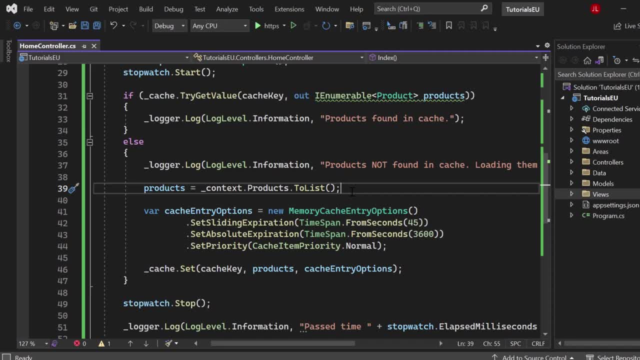 context Is not well working anymore. right dependency injection is working differently, So you have to make sure that you don't store the query. You have to store, well, collect. So the list, the array or whatever. That's why we say to list Now if you have no clue about the 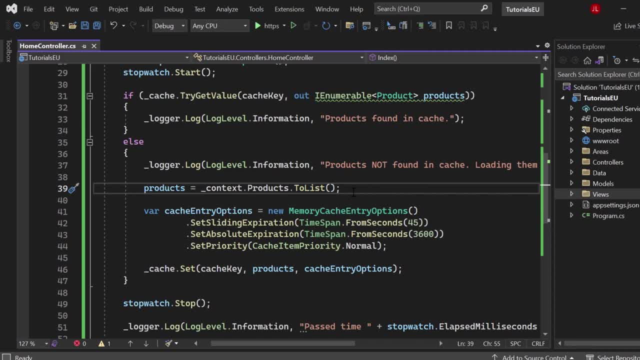 difference between an IQueryable and an IEnumerable. check out our video on that topic, since that's also very important for all ASPNET Core developers. Well, let me say that we really offer so much value for any NET developer out there. So, again, if you haven't subscribed to our channel, do it right now. 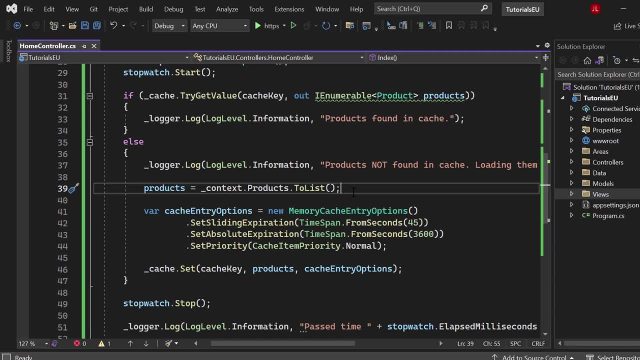 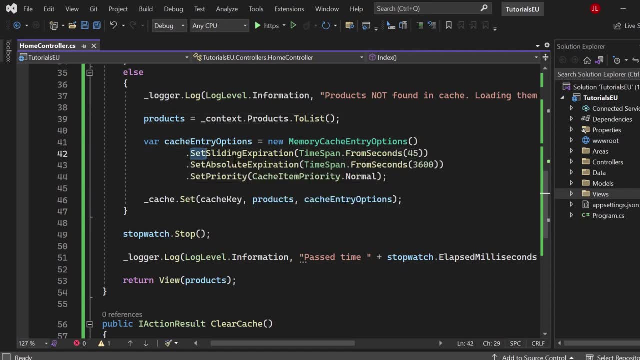 I'm absolutely sure that you will take amazing value from it. Now next up, we will dig deeper into the cache options. So we just create a memory cache, entry options. That's fine. And now we got three things here to set up. We got the set sliding expiration. We set it to 45 seconds. 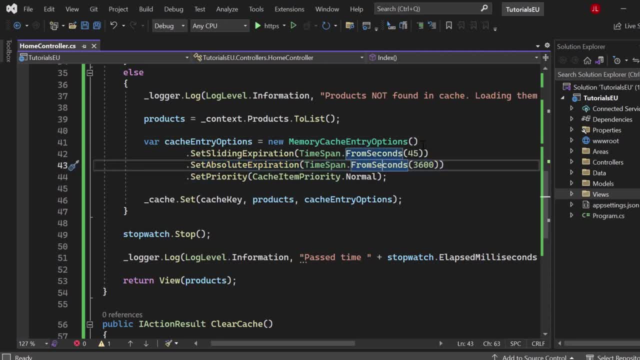 We've got the absolute expiration. We set it to 10 minutes And we got the priority and we set it to normal. Now let's dig deeper into that. So what is the sliding expiration? Well, let's assume that for sure, data changes in the database. 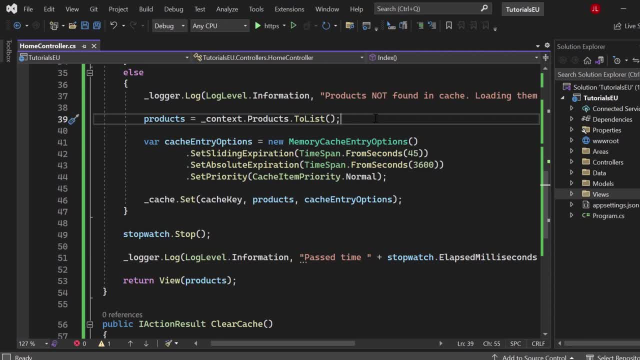 Right now, if we have an application that gets used by a lot of users, you don't want to store the data for too long Because, well, at any given time, you want to update the data, Right. So we've added new products and you for sure want to see those new products. So this is why we say like, okay, let's. 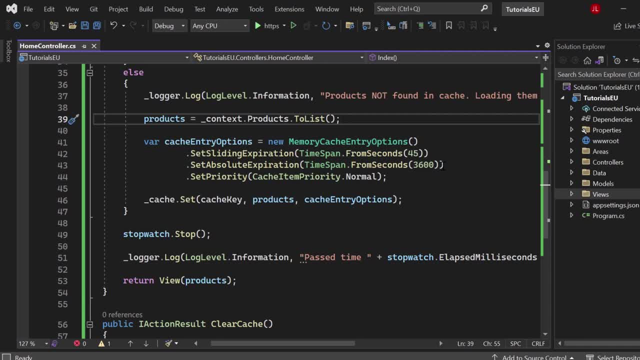 just save it 45 seconds. Something like that is really the industry standard, Something around 60 seconds Right, And after 45 seconds, if no one in the meantime has requested the cache, it will get cleared. So that means that this is sliding If after 30 seconds another user requests the cache. 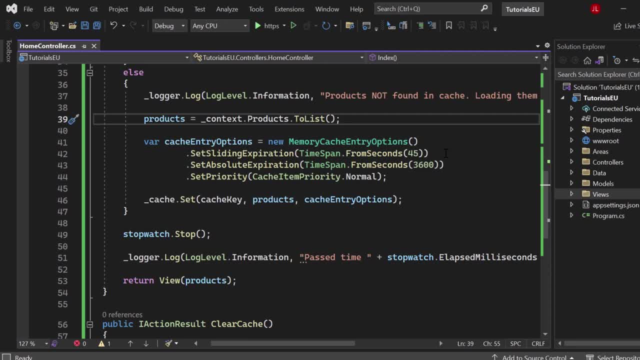 it will get set back to zero. Okay, That's the sliding expiration. Now for the absolute expiration. it doesn't really care about the sliding expiration. So, anyway, after 10 minutes the cache will get cleared, so that new created products will appear. Very important, Okay. So 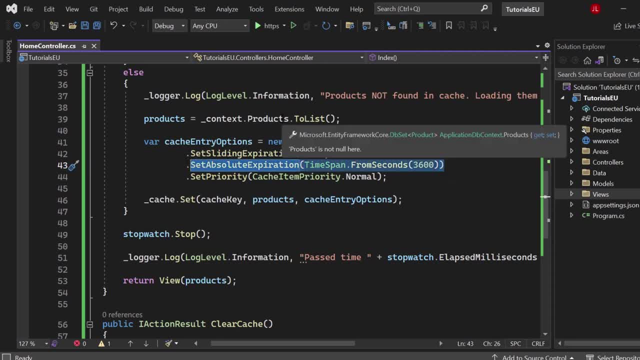 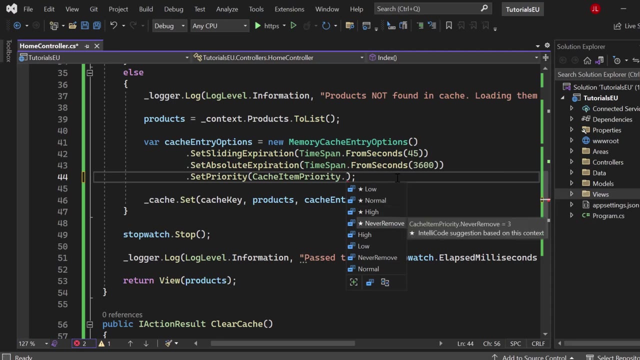 the absolute expiration is entirely independent from the sliding expiration, So after 10 minutes it will get deleted anyway. Now the priority is- let's just take a look here, That's easier to explain. We have low, priority, normal and high and never remove. So if we select, 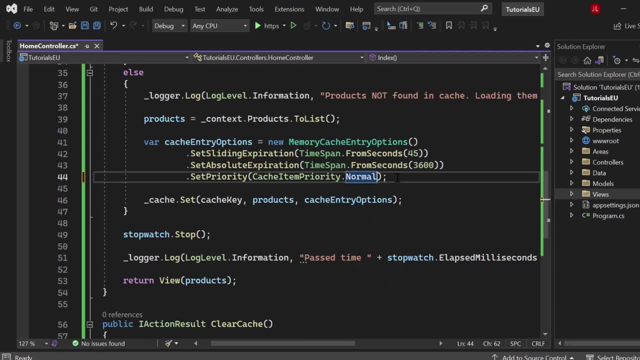 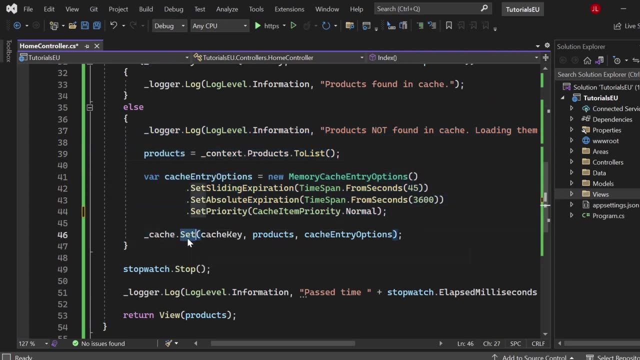 never remove. right here. the cache will never get removed, Right. So we simply set the priority to cache item priority, normal. Now afterwards, you can see, since we are here where products are not found, We are grabbing the products. We're configuring the cache. We simply set the element. 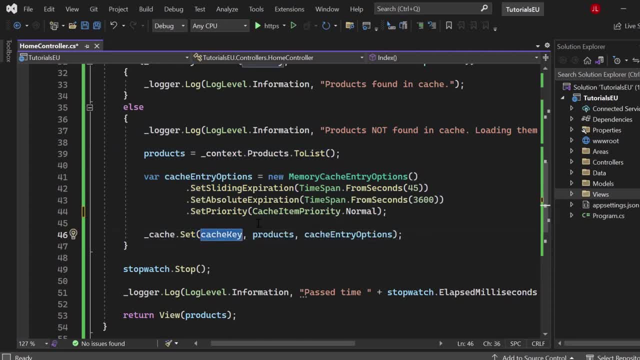 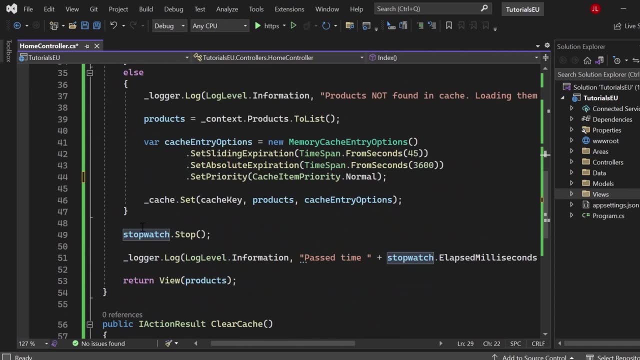 and then we save it into the memory cache. So we use the key again, We store the products, We submit our configured options. Now, here I stopped the watch right, So again here I started it. here I stopped it so that we can really see the delta time- Awesome. and then we just lock the information. 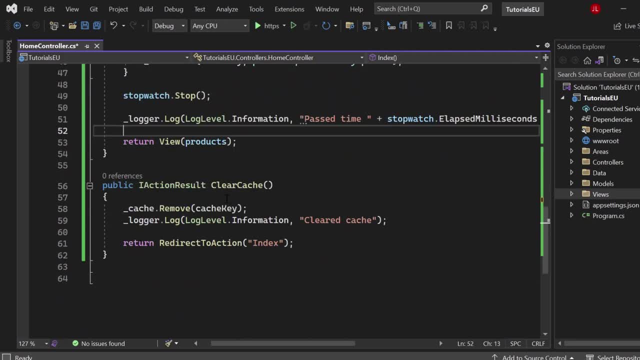 Return the view and see our data. Also, I created an action result, So a method that simply removes something from the cache. You simply take that cache object, call the remove method and submit the cache key so that you're able to follow the data. And that's it. That's the initial step. If you 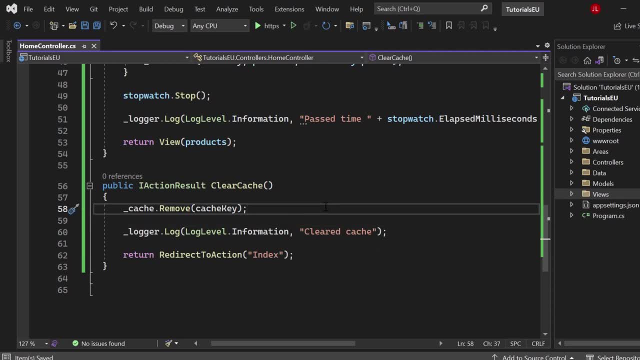 sure clear your cache. that's also something that you want to do. what you can do is if you add something new or delete something, um, like you add a new product or you delete a product, maybe you are interested in just immediately clearing the cache so that it's always fresh. keep that in mind. 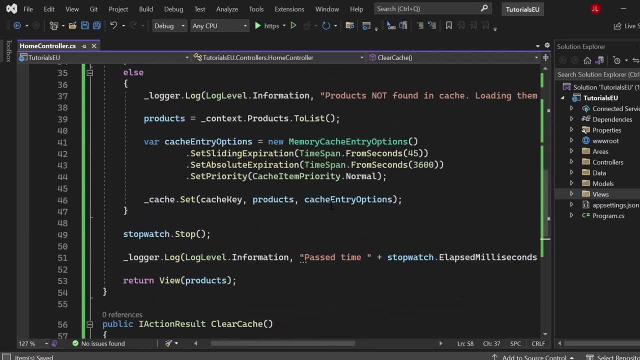 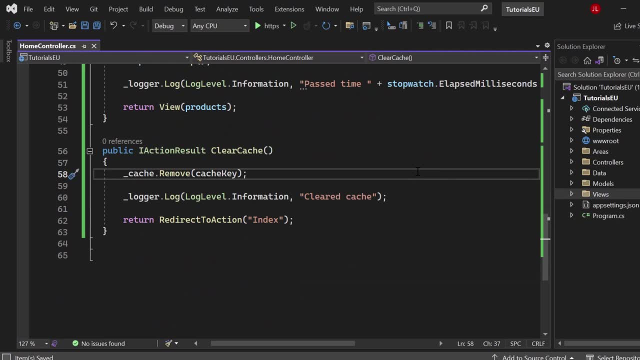 so this is basically what's going on here. now i want to point out- and that's very, very important- right, there is a possibility on running into a race condition, which basically means that if we have two users which are using the cache at the same time, chances are that they populate it, and 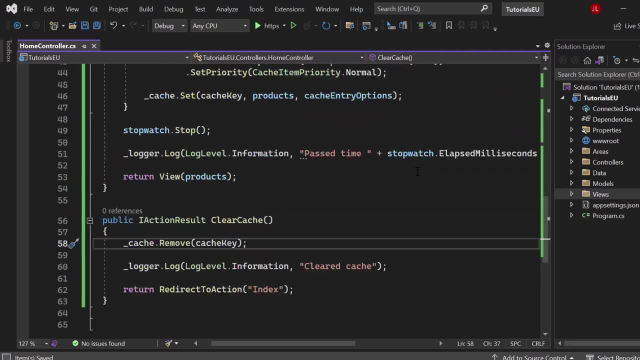 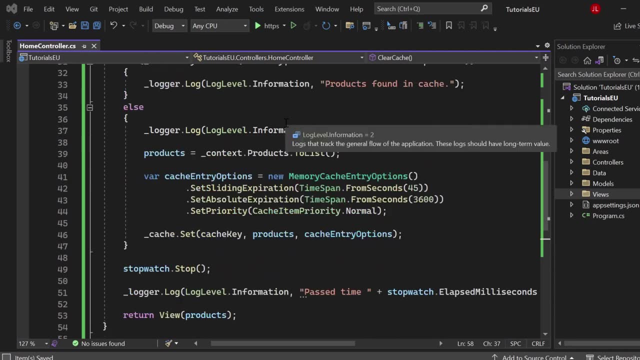 we run into that and we have a race condition. so what you'd have to do in that scenario is you have to create a lock to make sure that it's kind of thread safe, right. so if you're interested in seeing that, please write it down into the comment section below. i'd be happy to make another video on that. 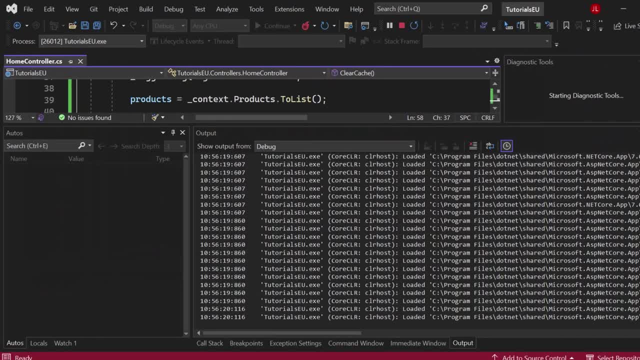 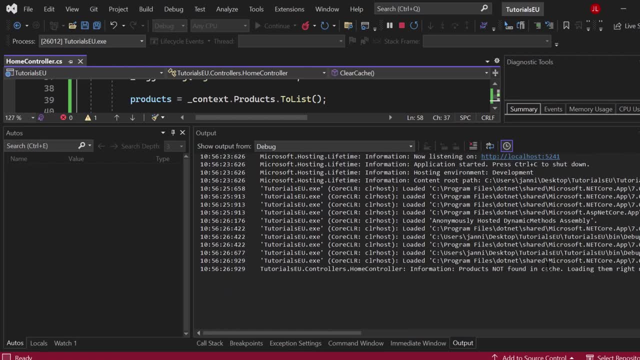 topic. now let's start our application one more time. let's just take a look at the debug log here. so it's starting and for sure a lot of time flies by right. we can see everything here. now is it's starting to look like a lot of time flies by right? we can see everything here. now is it's. 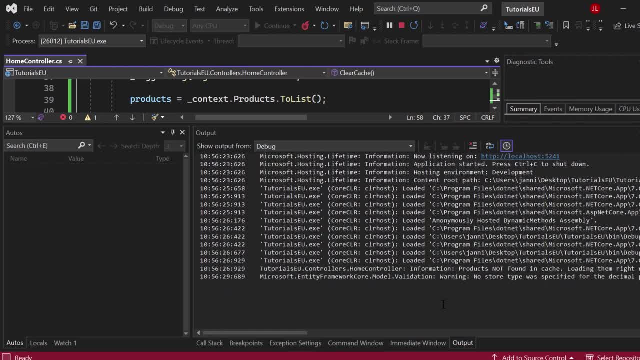 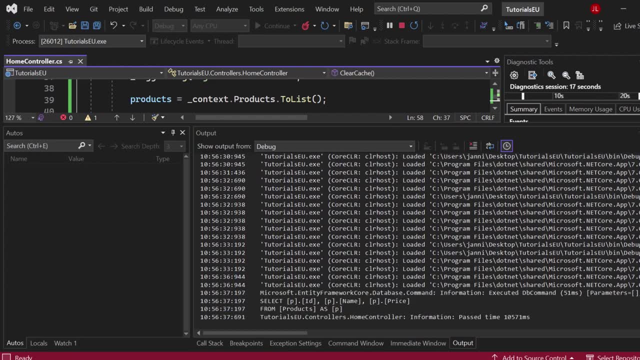 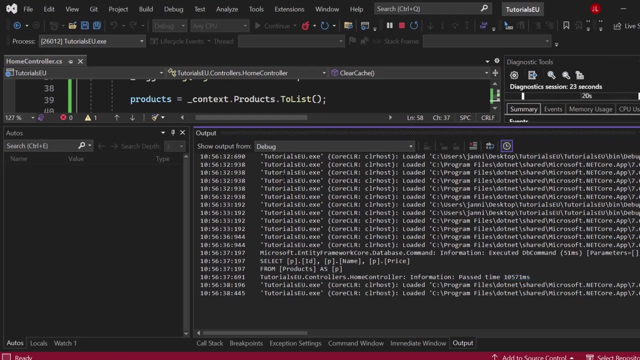 loading the stuff. the page gets loaded. it says: products not found in cache. loading them right now. blah, blah, blah. all of that takes really a lot of time. and on the other screen i can see that it's now showing up here. you can see like 100, uh, 10 000 milliseconds, but that's not the true value. 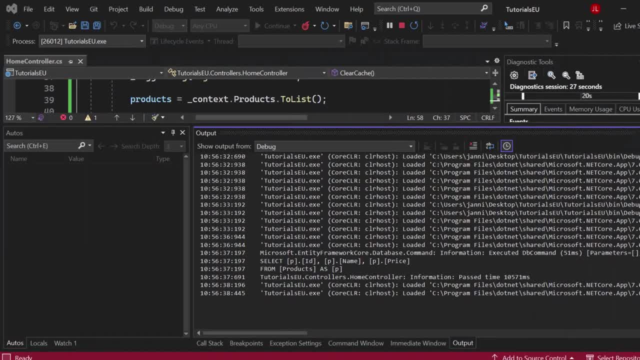 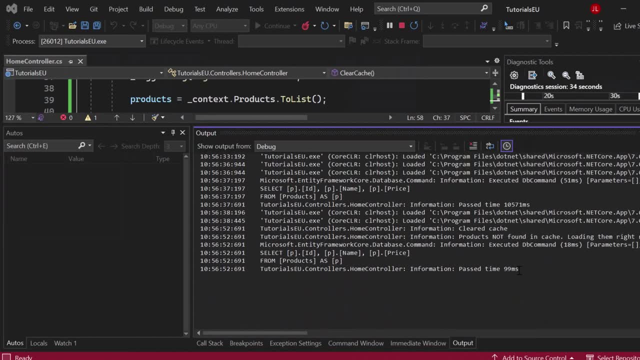 it took to only load the products right. so here we got our page. now let me just clear the cache. so i will simply click on clear cache so you can now see that the products got removed, cleared cache and it took 99 milliseconds to load them from the database and put them into the cache. 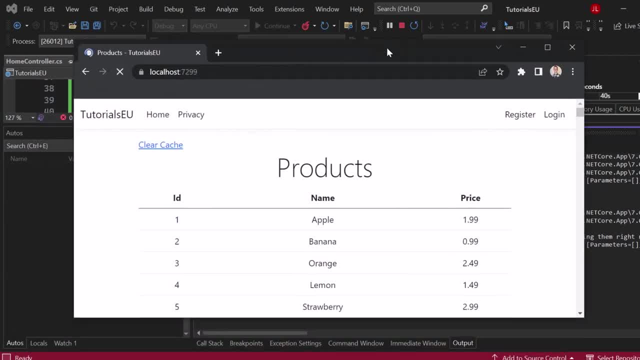 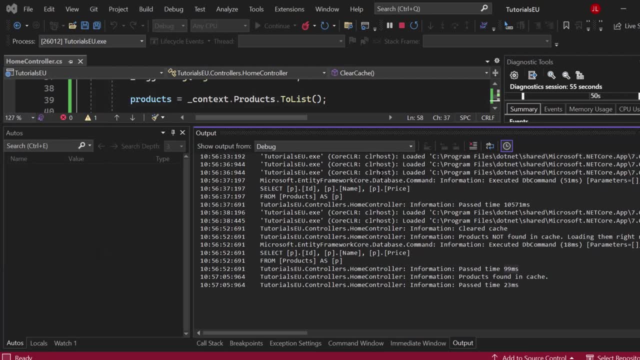 now, if i simply reload the page again, stuff will now get loaded from the cache, because 45 seconds- our sliding expiration time has not passed yet, so i'm loading it from the cache, and other users would do that too. you can see 23 milliseconds, which is a nice saving. 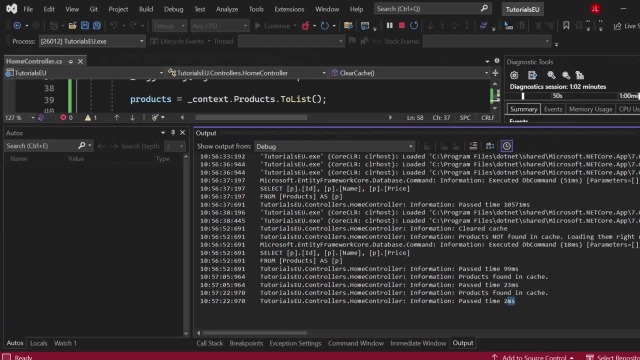 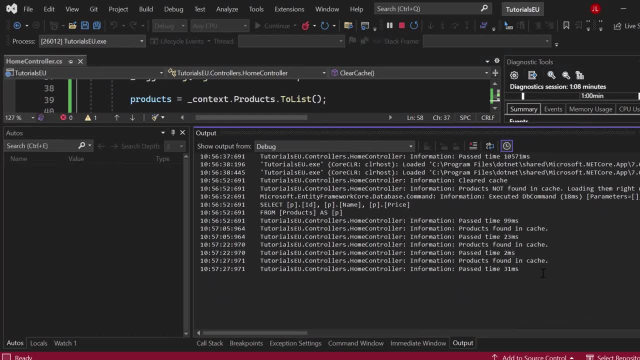 let's just try that again. how much time do we have now? two milliseconds, which is definitely awesome. 50 times faster, right? if i just reload it again, 31 milliseconds. anyway, you can see my screen recording software is really pretty watched up there. it really depends on the well. as i said, right now my computer is working quite.